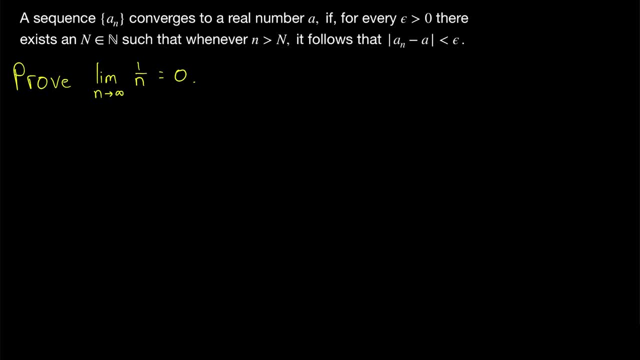 So I'll leave a link in the description to that lesson as well if you're interested. But for now we'll get our feet wet with the convergent sequence definition by proving this basic result For these convergent sequence proofs. I think it's pretty helpful to start. 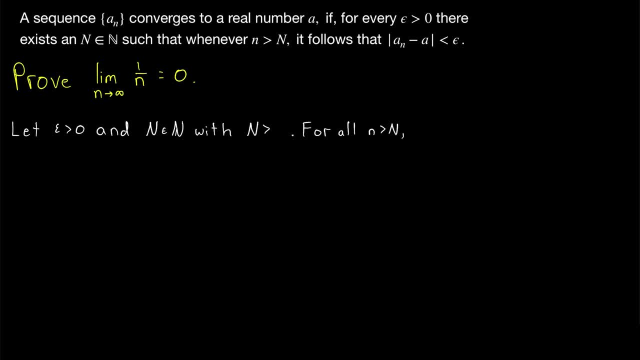 with a set of reciprocals of natural numbers that are equal to zero. If you're interested, you can start off with a sort of template guiding us in the right direction of how this sort of proof will go. We know we're going to take some arbitrary epsilon greater than zero. Then we'll 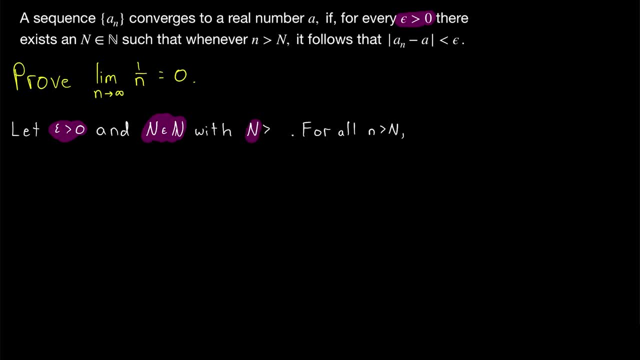 have a natural number, big N, that is sufficiently large so that for every term of the sequence after the big nth term we have that the distance between those terms of the sequence and the supposed limit, which is zero in this case, that distance is less than. 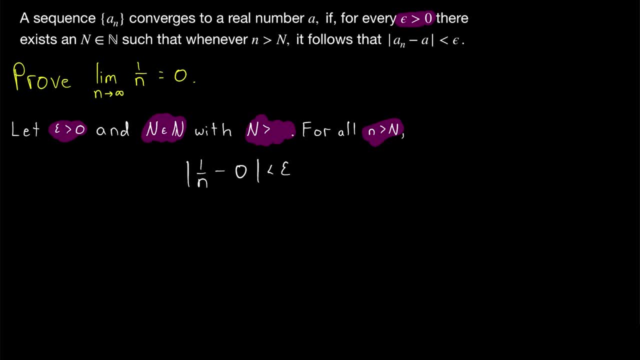 epsilon. Of course, our primary challenge is figuring out how big big N has to be and then showing that that will indeed work. I think it's a good idea to start off with this key expression: the distance between terms of the sequence and the limit. And for starters, 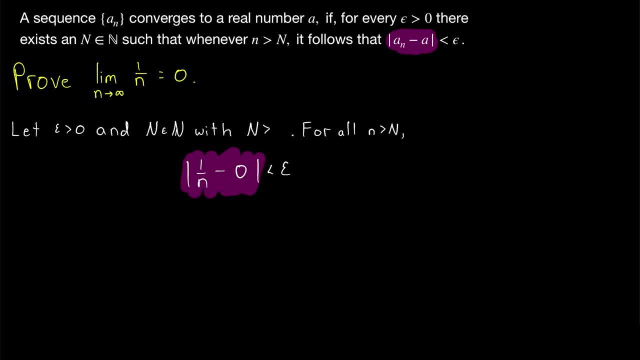 just see what simple simplifications we can make to the expression. Remember, our proof really ends with less than epsilon, so let's forget about that for now and just focus on simplifying the expression. The first thing I notice is that minus zero doesn't do anything, so we know this. 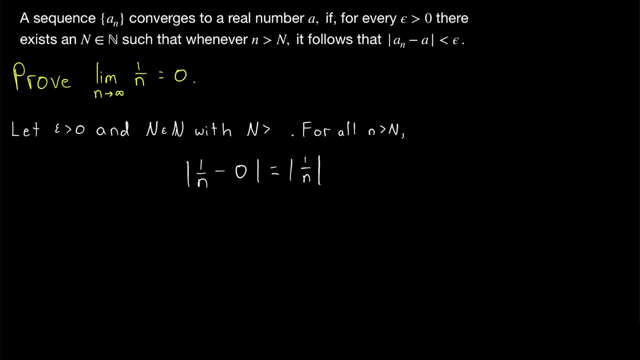 is equal to the absolute value of 1 over N. But then when we're talking about a sequence like 1 over N, remember N is a natural number, like 1,, 2,, 3,, 4, and so on. Every natural number is positive. 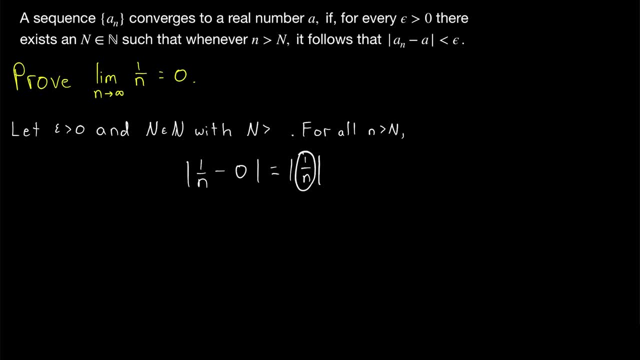 which means that 1 over N is always positive, which means these absolute value bars aren't doing anything. So this is equal to 1 over N without the absolute value bars. So now we've done some basic simplification. We know that we want this to be less than epsilon. How are we going to get there? 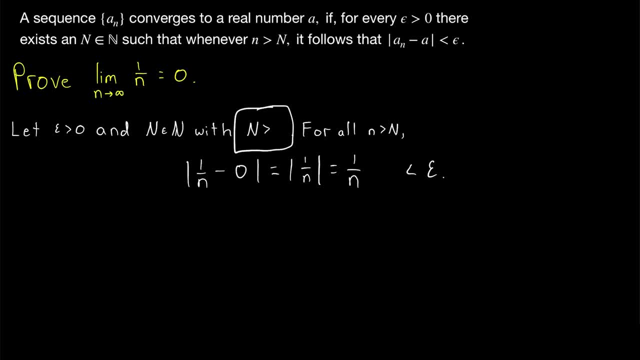 This is where we are going to figure out how big big N has to be. We're basically just going to do some scratch work that wouldn't actually have to be in your proof, but you'd have to do it to figure out how to write the proof. We want 1 over N. 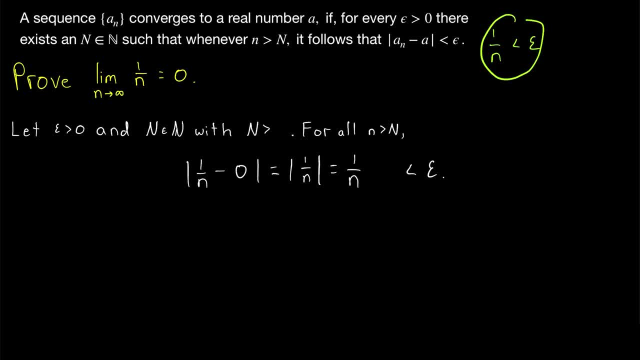 to be less than epsilon. so we just want to solve this inequality for N, to figure out how big it has to be to make our desired inequality true, Because, remember, N can be as big as we need it to be. We can go as far along in the sequence as we need to to make sure that this distance is less. 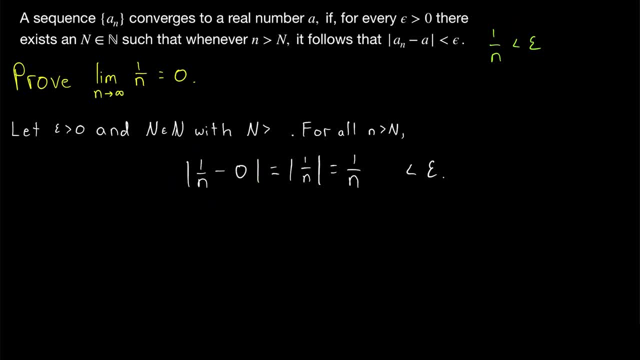 than epsilon. To solve for N here: well, right now we just have 1 over N, so all we have to do is invert both sides of the inequality. To solve for N here: well, right now we just have 1 over N, so all we have to do is invert both sides of the inequality. 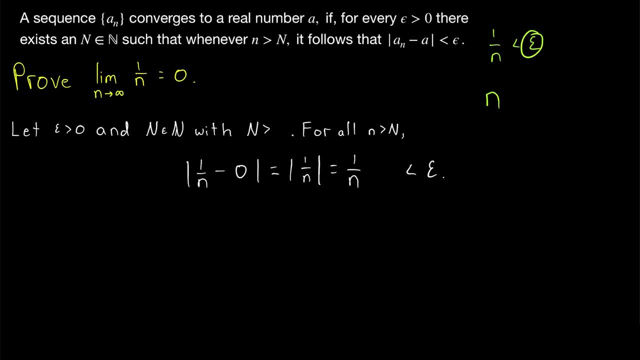 Doing that gives us n on the left side. and then inverting epsilon gives us 1 over epsilon on the right side. And remember, when you invert both sides of an inequality you've got to flip the inequality So less than becomes greater than. 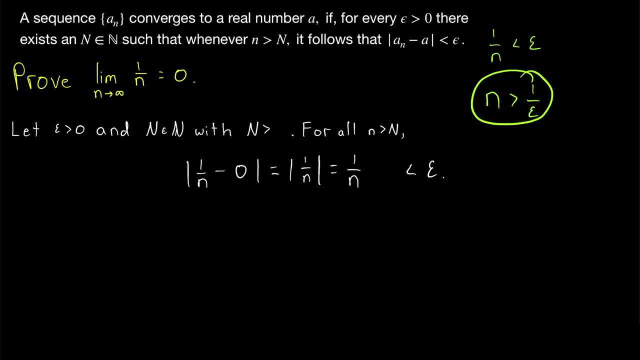 So we need n to be greater than 1 over epsilon. So since n is greater than big N, if we make big N greater than 1 over epsilon, we should be good to go Now, when you're still early on in your real analysis course. 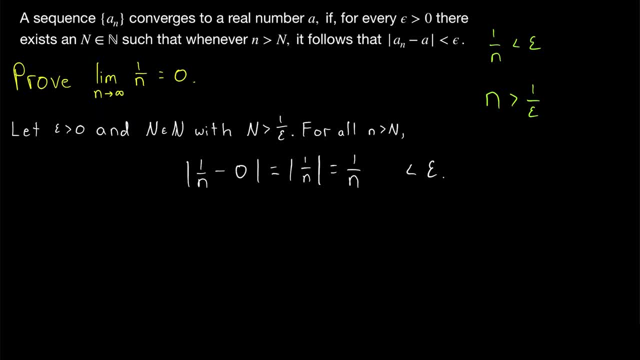 which you probably are. if you're proving this result, it's probably worthwhile to add in your proof that we know a natural number this big exists by the Archimedean Principle. I'll leave a link in the description to my lesson proving the Archimedean Principle. 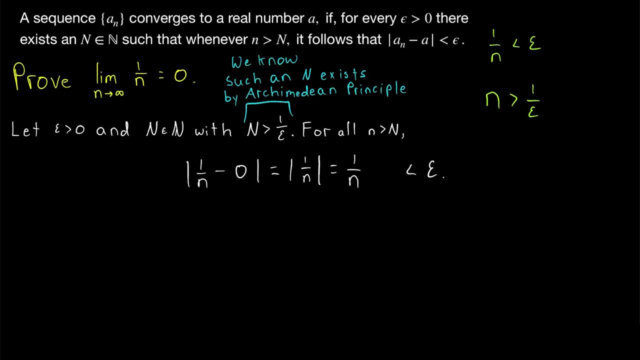 and it's sometimes stated in a few different forms, But in short, it tells us that for any real number we can find a bigger natural number. So that's how we know that we can find this natural number, big N, that's greater than 1 over epsilon. 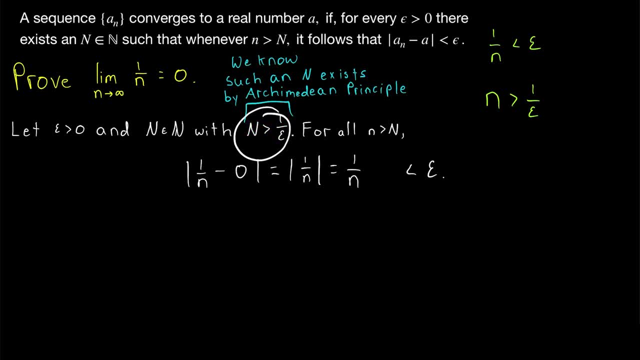 Now we can finish our proof. We figured out how big big N has to be. Now we've got to fill in the holes to show that works. Remember that we took n to be greater than big N. So if we replace n here in the denominator with big N, 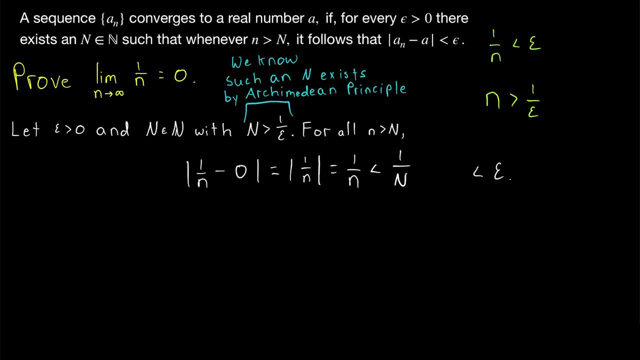 that will give us a bigger number. And again, that's because n is greater than big N. So here 1 is being divided into fewer pieces than it is over here, which is why we have a bigger number. Anytime we divide by a smaller number, the quotient gets bigger.